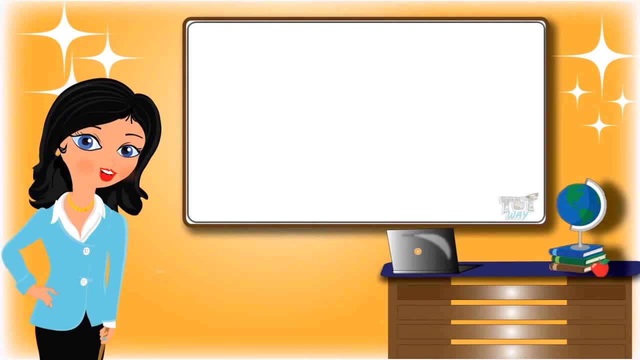 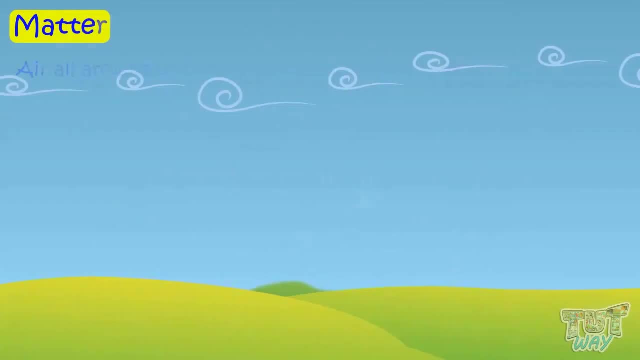 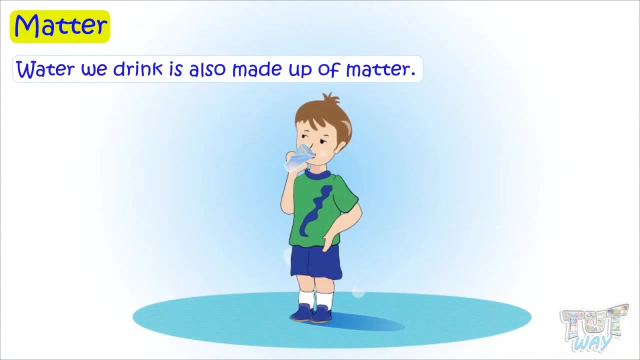 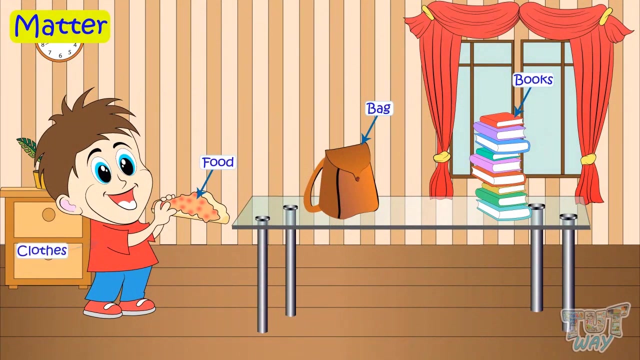 Hi friends, Today we will learn what is matter. So let's start. Air all around us is made up of matter. Water you drink is also made up of matter. Your books, your bag, food you eat, clothes you wear are all made up of matter. 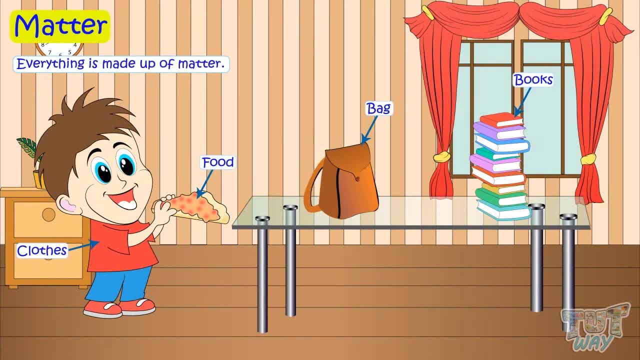 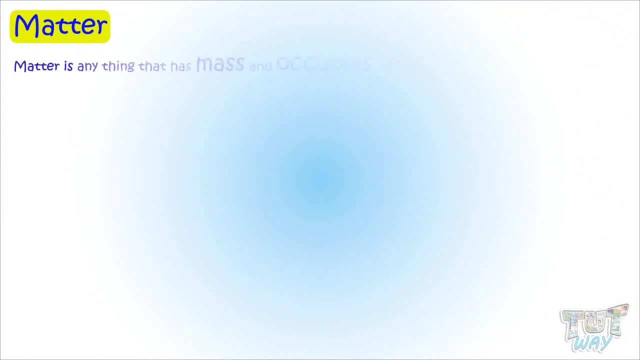 or just everything you see all around is made up of matter. Definition of matter is: matter is anything that has mass and occupies space. Now let's understand this definition. First point is: matter has mass. It means matter has some weight. Second point is: it occupies space. 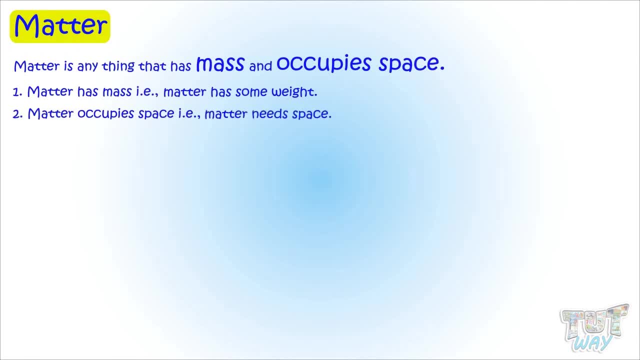 It means matter has some weight. Second point is it occupies space. It means matter needs space. Let's take an example to prove it. We learned that everything is made up of matter. So let's take a few things and see: are they made up of matter? First is water. We have to see if water is made up of matter. 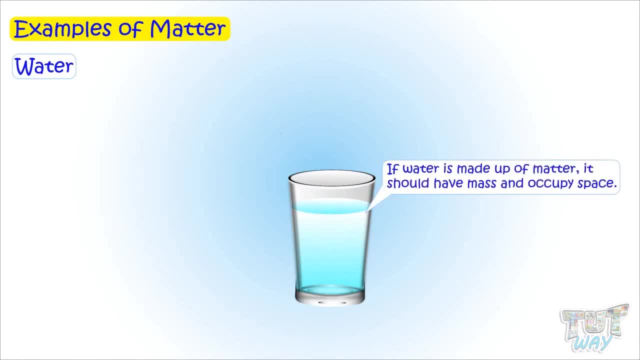 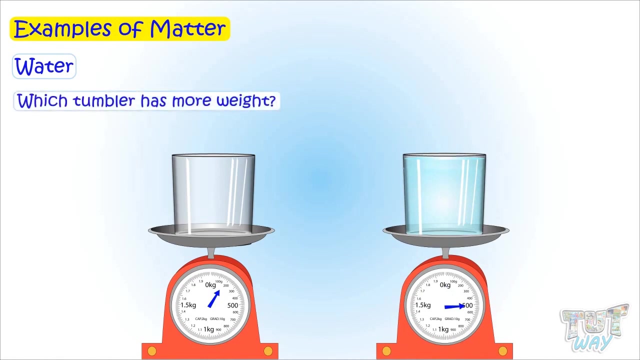 It should have mass and occupy space. Take an empty tumbler. Take an empty tumbler and weigh it. Now fill it with water and again weigh it. Which tumbler has more weight? The filled tumbler has more weight. 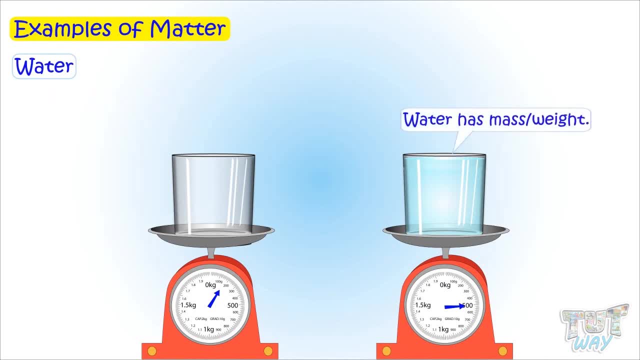 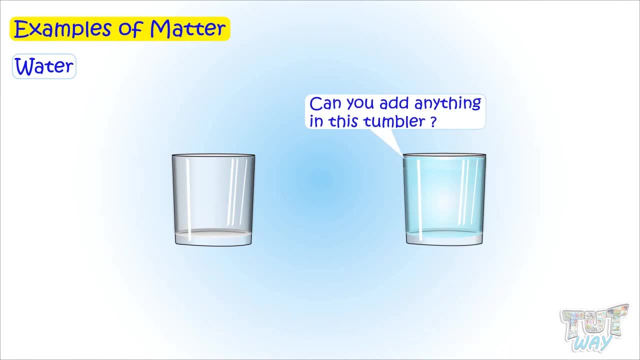 It means that water has mass or it has weight. Now, can you add anything to a tumbler which is already full? No, you cannot add anything to a tumbler. You can't add anything to a tumbler which is already full. You can't add anything to a. 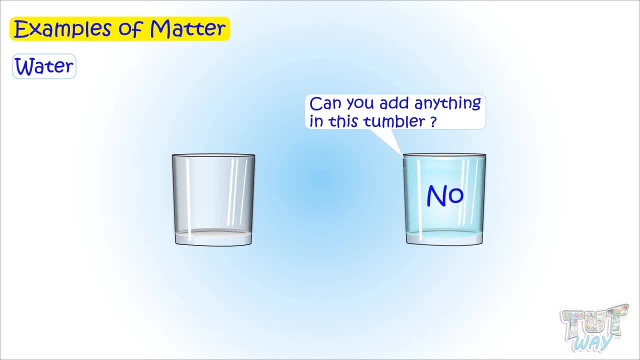 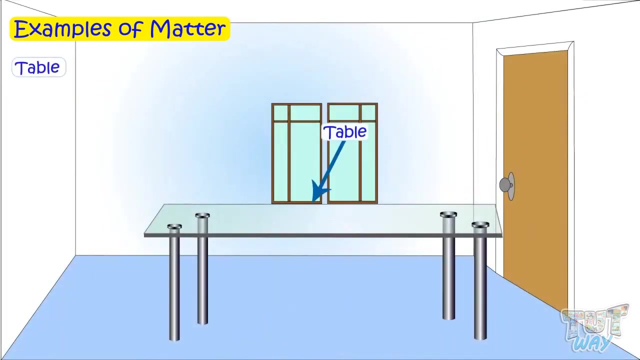 tumbler which is already full with water or any other liquid. So it means that water or any liquid occupies space. So water or any liquid has mass and occupies space. So it is matter. Now here is another thing and it is a table. We have to see if this is made up of matter. 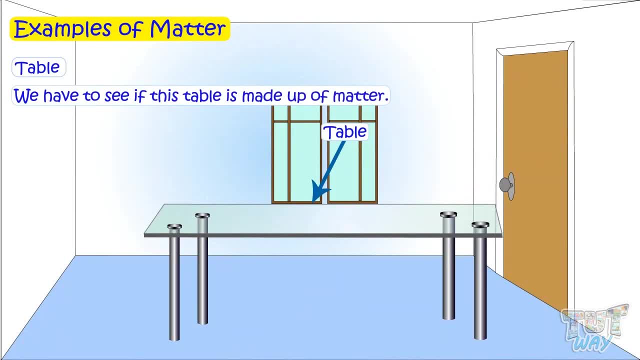 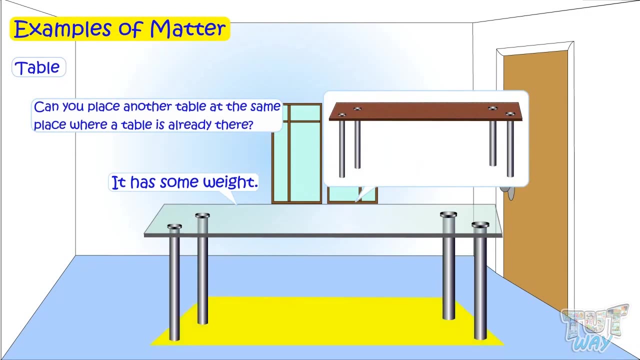 and for that we have to prove It has mass and it occupies space. Weigh the table. It has weight. Now can you place another table at the same place where a table is already there? No, you cannot. So table occupies space. 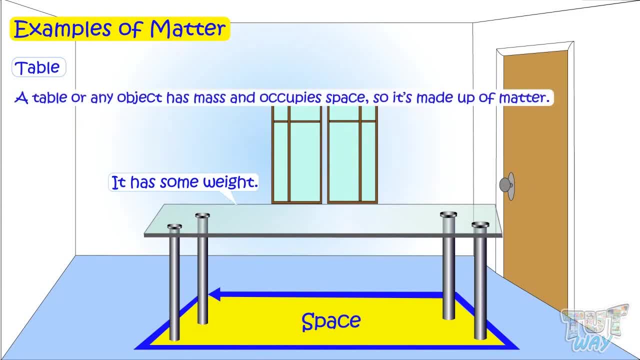 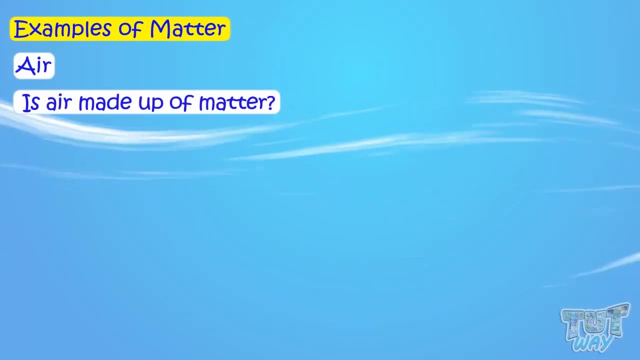 So table or any solid object has mass and occupies space, So it is made up of matter. Now we will see whether air is made up of matter, And in order to prove that air is made up of matter, we should be able to prove that air has mass and occupies space. 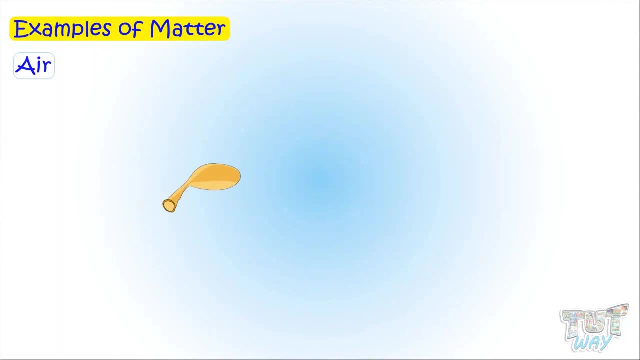 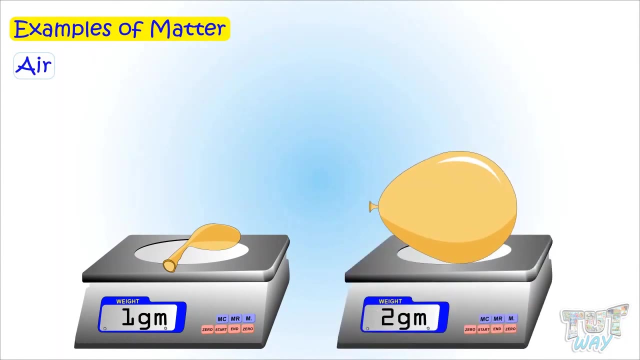 Now take an empty balloon and weigh it. Now fill the same balloon with air. again weigh it. Which balloon has more weight? Filled balloon will have more weight. It means that air has mass or it has some weight. Now let's see if air 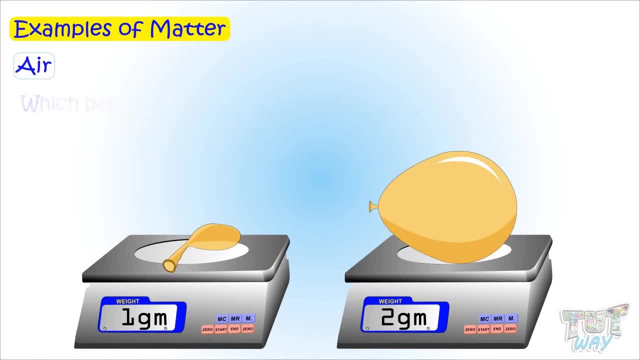 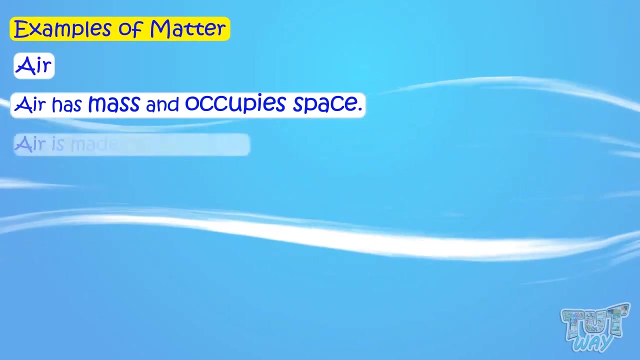 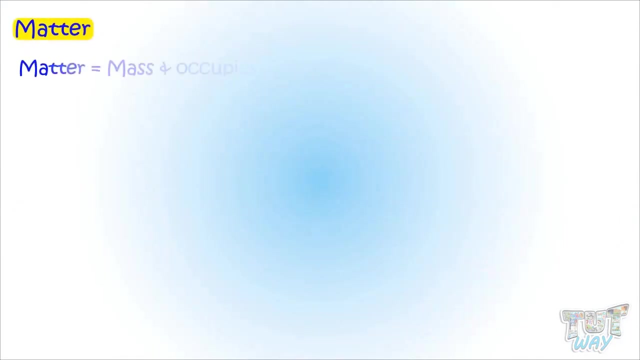 occupies space. Now, which balloon occupies more space? A empty balloon or a filled balloon? A filled balloon occupies more space. so it means that air occupies space too. So air has mass and occupies space. So we can say: air is made up of matter. So kids, now we know matter is anything that has mass and occupies. 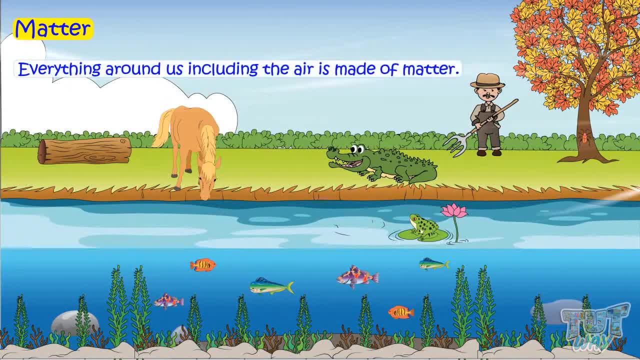 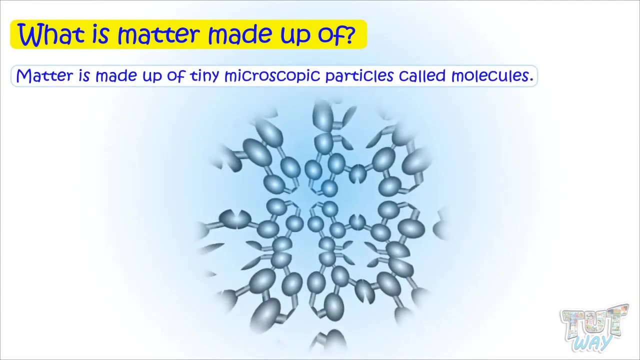 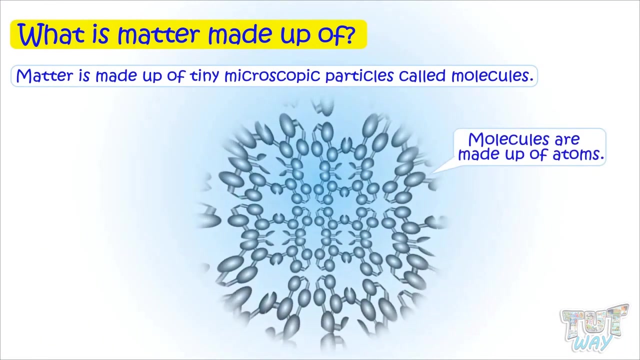 space and everything around us, includes the air, is made of matter. Now we will see what is matter made up of Matter. Matter is made up of tiny, microscopic particles called molecules, and further molecules are made up of atoms. The density in the space between particles. 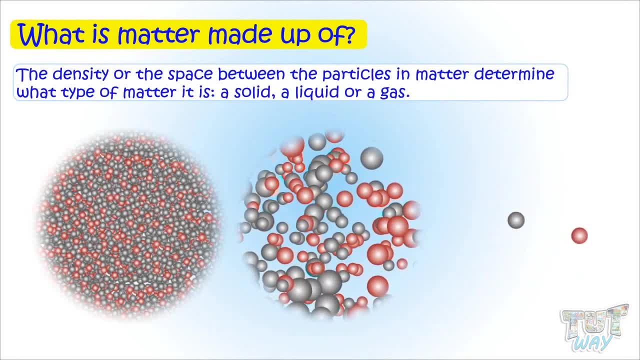 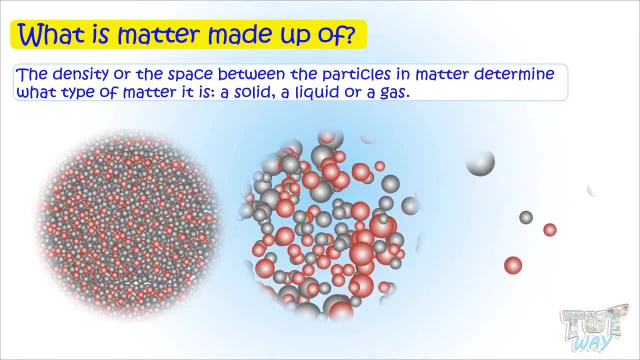 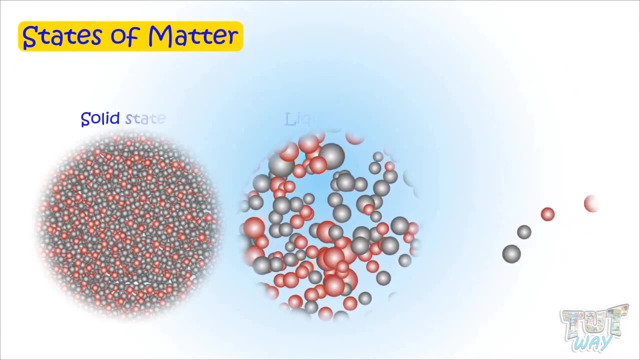 of matter determine what type of matter it is. The density in the space between particles of matter determine what type of matter it is: solid, a liquid or a gas. So states of matter can be solid, liquid or gaseous depending on the density and 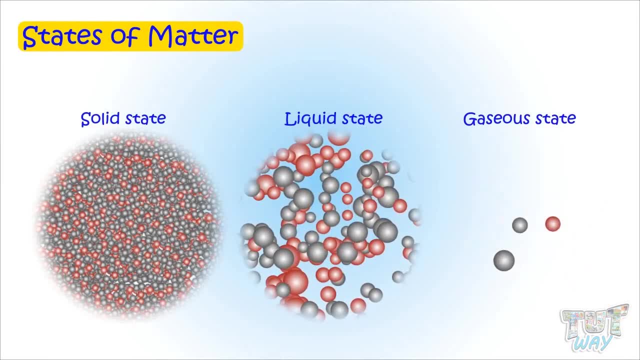 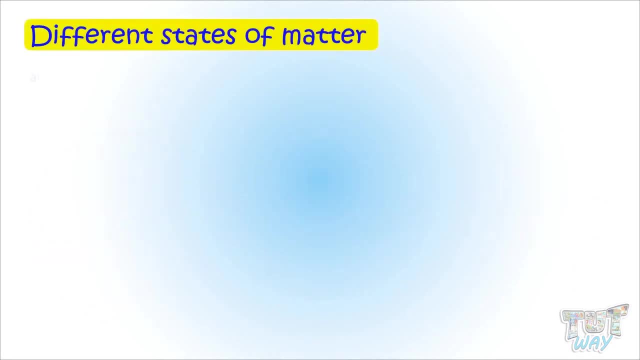 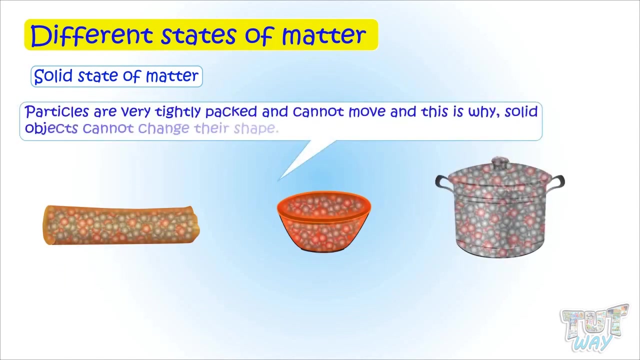 the space between the particles of the matter. Now we will learn about the different states of matter: Solid, liquid and gas. First let's learn about the solid state of matter, The matter that is a solid state, like wooden objects, plastic objects and steel objects, The particles are very tightly packed and 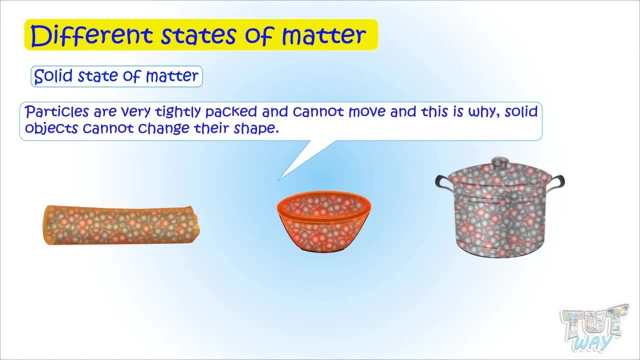 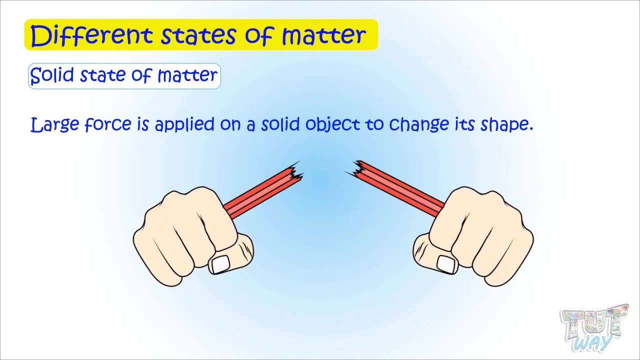 cannot move at all, and so that is why matter is solid. Solid objects cannot change shape and remain in the same shape unless large force is applied on a solid object to make it change its shape. Next we have liquids. Liquid objects like water, juice, milk or just any liquid. 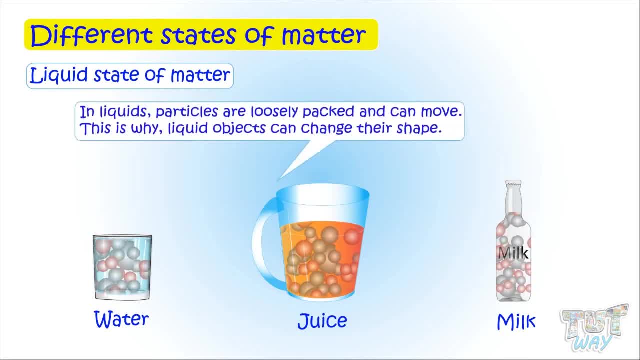 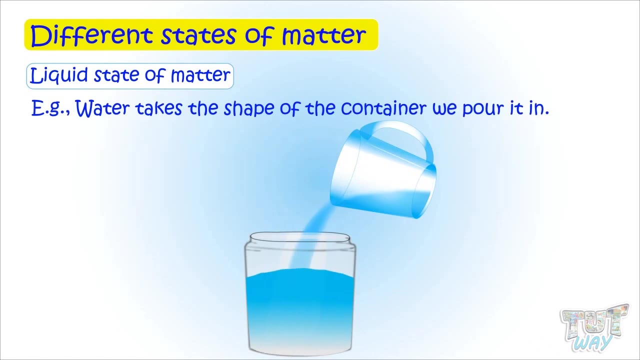 particles are loosely packed and can move. This is why liquid objects can change their shape. Example: water takes the shape of the container we pour it into. And if we pour water in a glass, shape of water is same as that of the glass. If you pour the 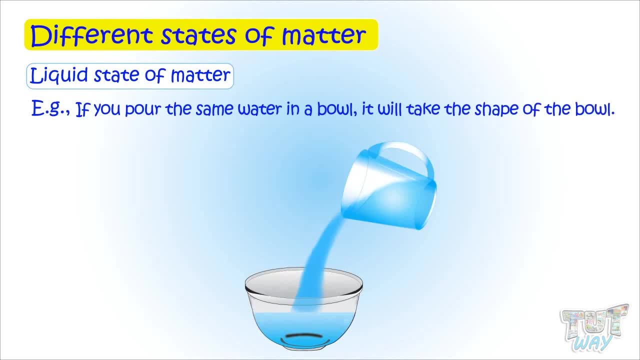 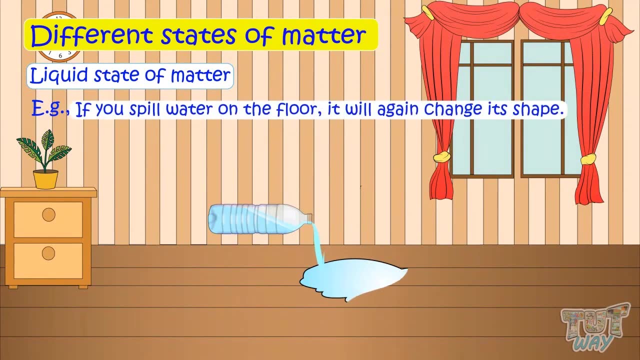 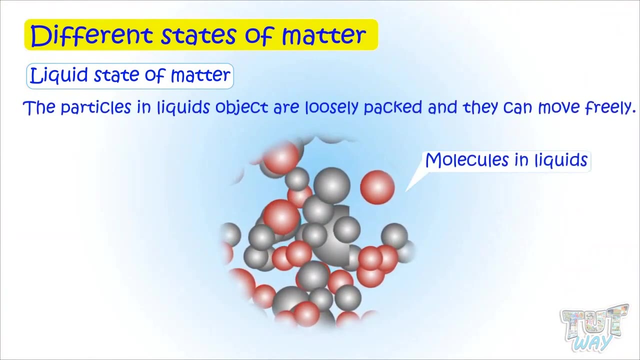 same water in a bowl, it will take the shape of a bowl, And if you spill water on the floor, it will again change its shape. This is all because the particles in a liquid object are loosely packed and they can move freely. 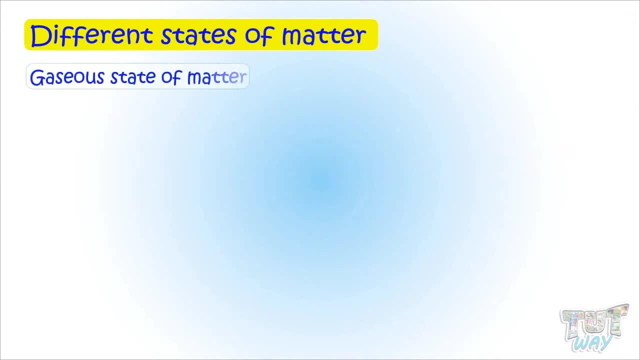 Now, third form of matter is gaseous state. In gaseous objects like air, perfumes, steam, particles are very, very loosely packed, Even much more loose than the liquid, and can move very freely, And so that is why gaseous objects do not have any shape. 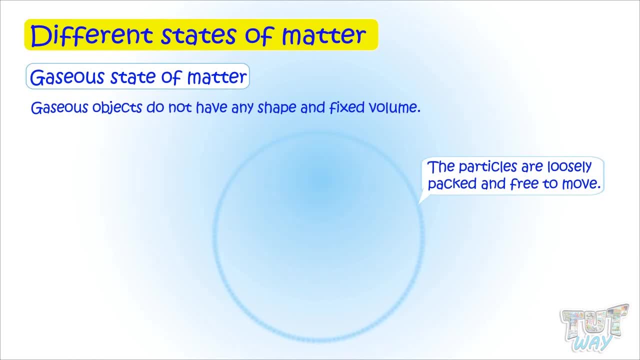 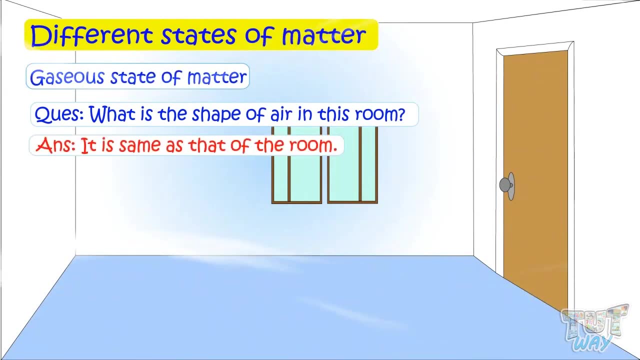 They take the shape of their container. What is the shape of air in this room? It is the same as that of the room. What is the shape of air in this balloon? It is the same as that of the balloon. It is the same as that of the balloon. 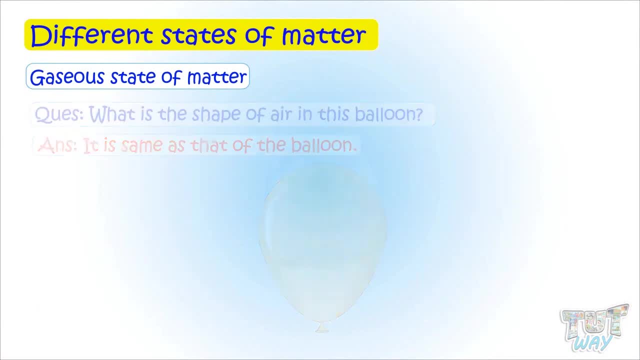 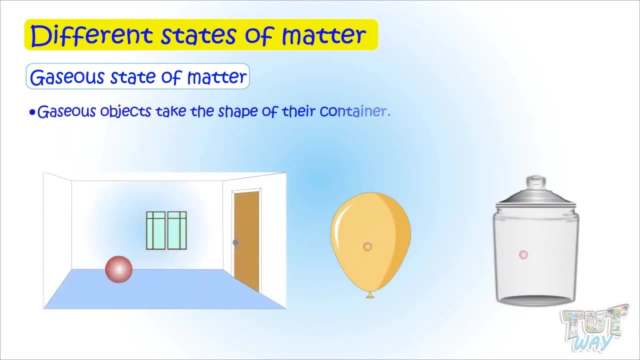 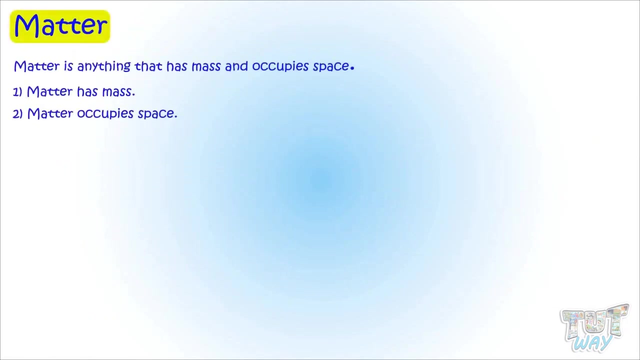 And so that is why gaseous objects do not have any shape. They take the shape of their container and they do not have even a fixed volume, as the particles are very loosely packed and they are free to move. So, kids, today we learned what is matter. 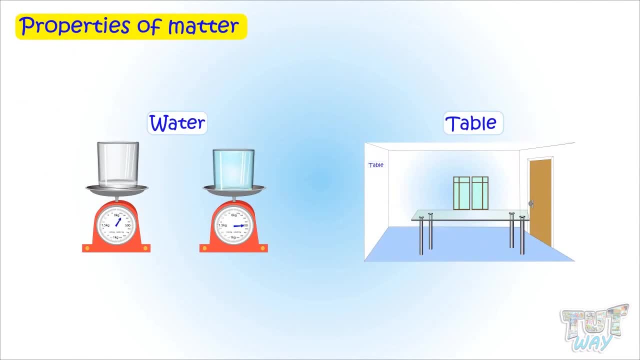 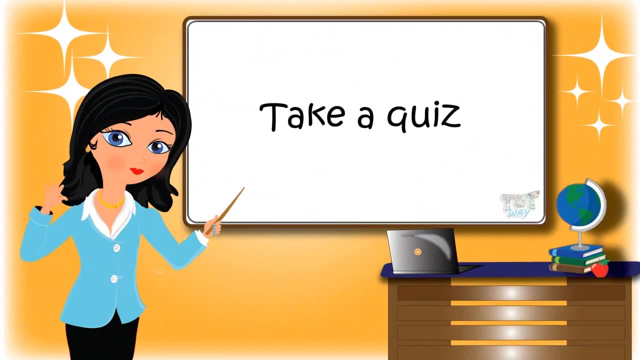 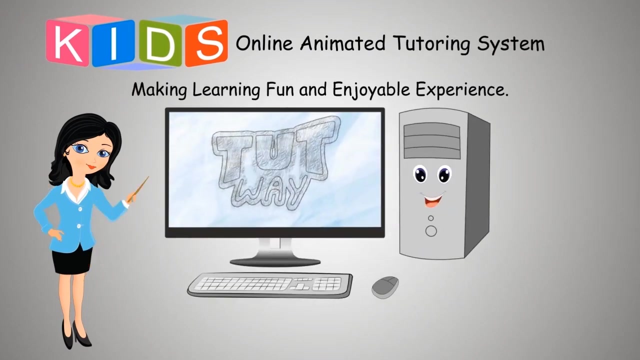 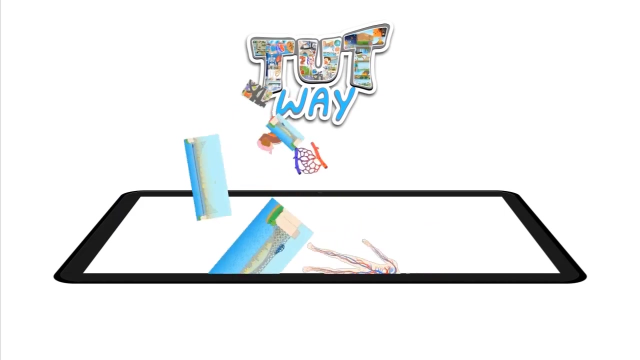 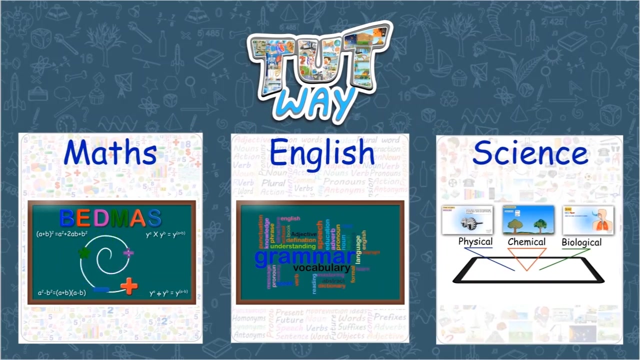 properties of matter and different states of matter. Okay, kids, now you may go ahead and take a quiz to learn more. Bye, bye. TootWay has thousands of animated videos on math, English and science to clear the core basics of these subjects. 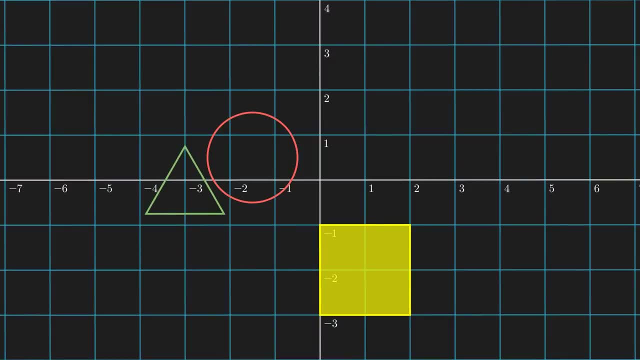 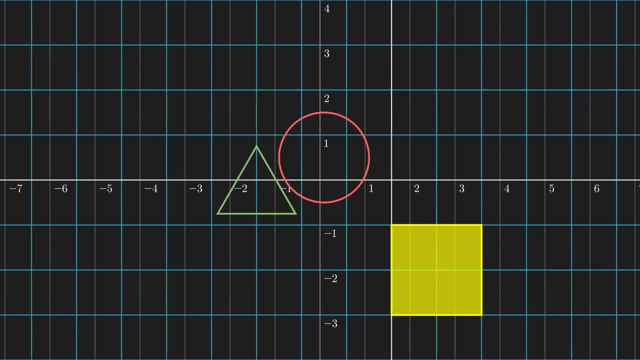 While I was working on another video, the topic of special Euclidean group came up, which, roughly speaking, is a collection of all translation and rotation in space, And translations and rotations do not commute with each other. If we translate two steps to the right, then rotate 90 degrees about the origin. 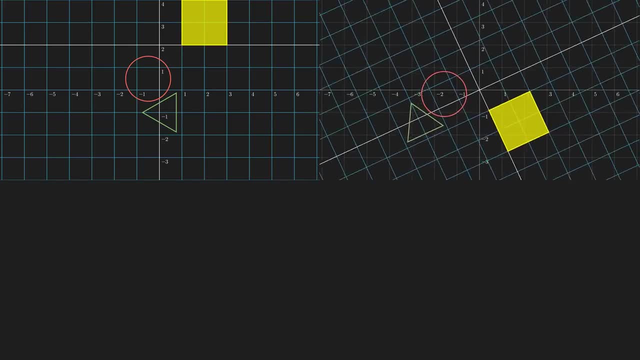 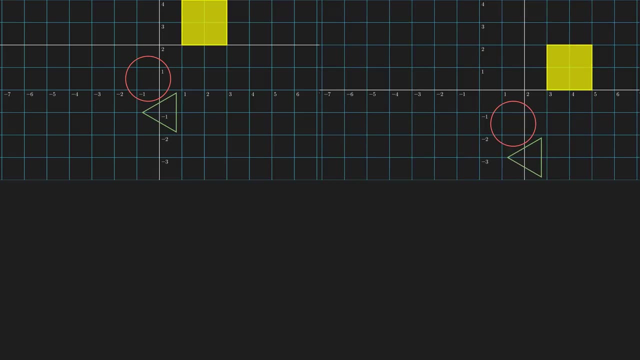 then we would get a different result. if we do them in reverse, which is to rotate first, then translate two steps to the right. Now the real interesting thing is: either way we compose these transformations, they end up being rotations about some other point in space. 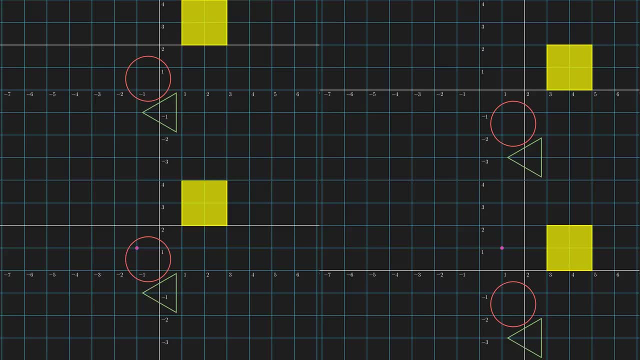 And that raises couple of questions. Why did they end up being rotations about some other point, which is and, respectively? And the more important question is: can we come up with a formula for rotating about any point in space? And we will see in this video how that very technique that we are about to